So how can you do that? You need to fine tune 3y minus 3 y Because, as you understood, 3y-3y equals 0. But why missing 4x, which is the fourth day on the right, If 3y-3y equals 0, you need to be careful, because truing will produce more, called truing problems. 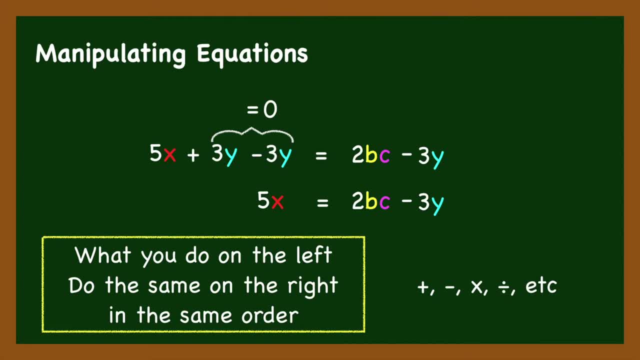 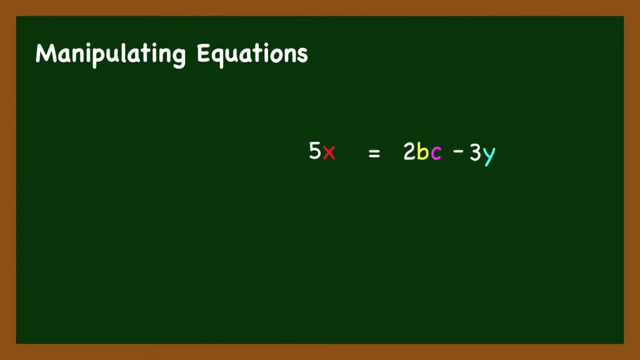 Because maybe in practice you will learn to make all three segments equal: your addition, subtraction, multiplication, division or whatever operations that you need to perform. Now let's finish this equation by finding x, which is the usual question anyway. So again, what you do on the left, do the same on the right, in the 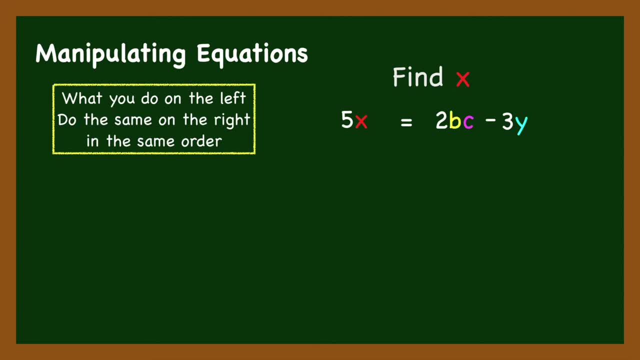 same order. To isolate x, I just need to divide the left-hand side by 5, but since I did that for the left-hand side, I need to do that for the right-hand side as well. Now, 5 over 5 is equal to 1.. So effectively, that leaves me with x, and now my equation becomes x equals. 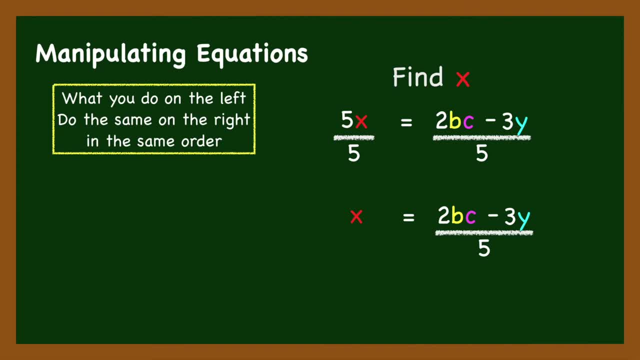 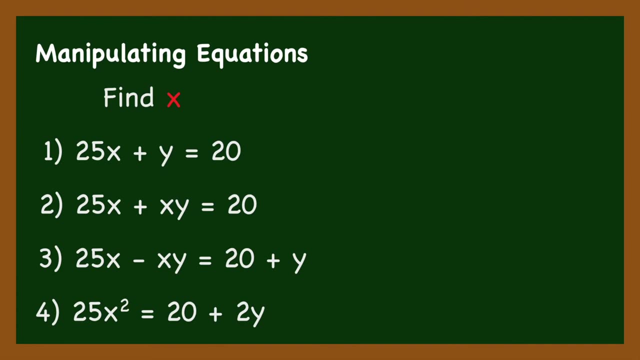 2. 2bc minus 3y over 5.. And that is my answer. Now let's practice with some equations. Can you find x in these equations? Pause this video now and solve it. So let's take the first equation: 25x plus y equals 20.. Can you guess what I'm going to? 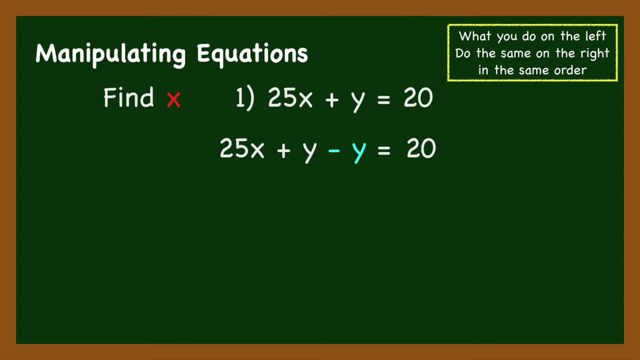 do next? I will just subtract y on both sides. That will give me 25x equals 20 minus y, But I'm still not done yet. So, just like with our example, I just need to divide both sides by 25, and that will. 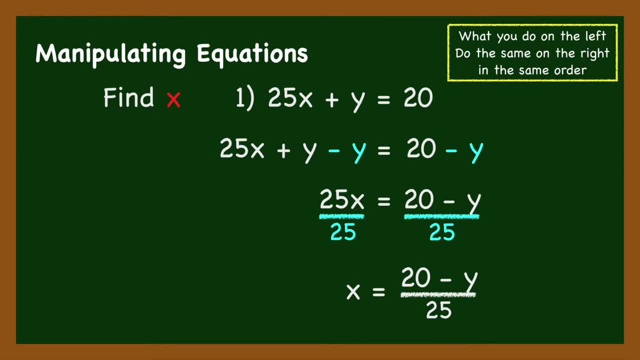 give me, x equals 20 minus y over 25.. Second question: 25x plus xy equals 20.. Now here's a trick that I will do: I will factor out x And multiply it by 25. And multiply it by 25 plus y, Which is equal to 20.. 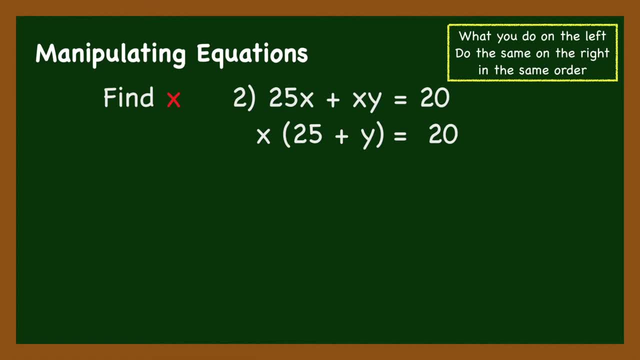 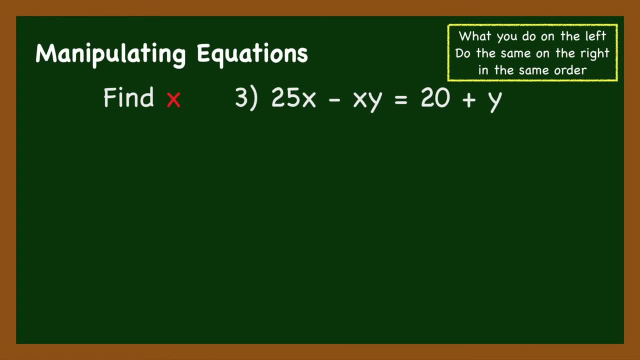 That will leave me with this answer: x equals 20 over 25 plus y, again with a slightly different question. so now we have 25 X minus X. Y equals 20 plus Y. so first step, I will factor out X. so now it's X times 25 minus Y, which is: 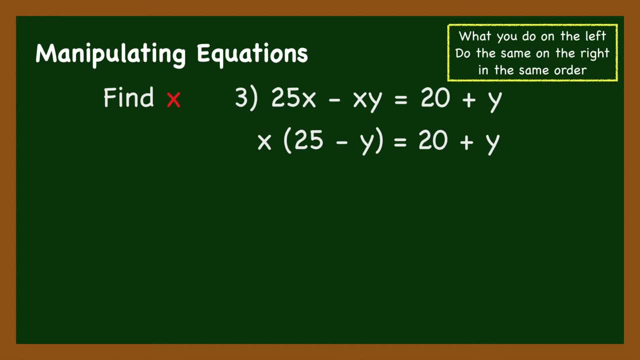 equal to 20 plus Y. so what will I divide both sides with? so I just divided by 25 minus Y and I get my answer: X equals 20 plus Y over 25 minus Y. are you having fun so far? I hope you're starting to find it easy. now let's go to the fourth.